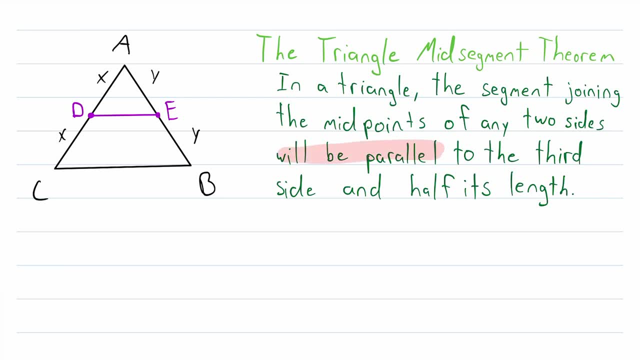 that two segments are parallel and we're trying to prove that the length of one segment is half the length of another segment. Notice that half is a ratio: the ratio 1 to 2.. When we're talking about triangles and ratios- a concept that should immediately come into- 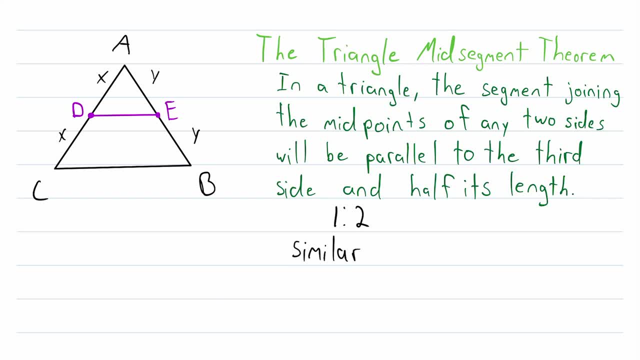 your mind is the idea of similar triangles. Of course, to talk about similar triangles, we need two triangles. Do we have two triangles in this situation? Well, we certainly do. We have the original triangle ABC and we also have this triangle AED. So if we could, 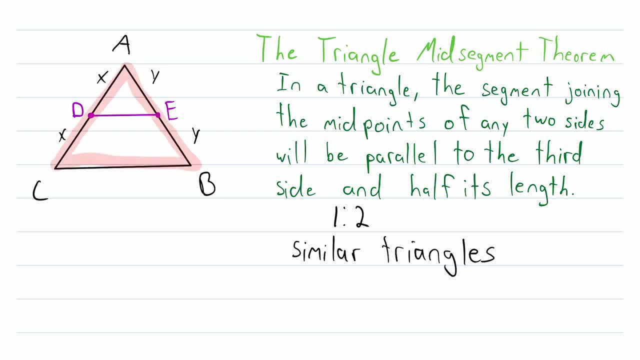 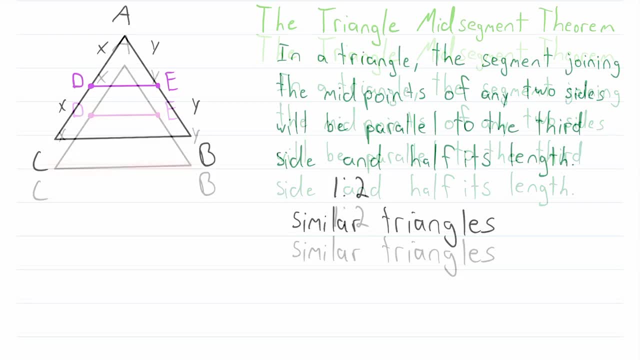 show that AED is similar to triangle ABC, we might have a shot at showing that this line segment is half the length of this line segment. And if we were to go back to the argument and if we're observant, we may immediately notice that the side AD is half. 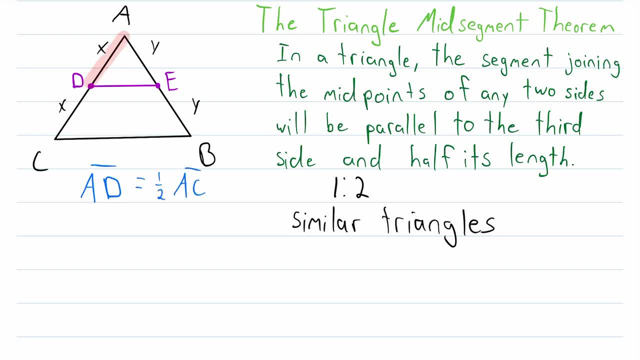 the length of the side AC. That's because AD has a length of X and AC has a length of X plus X, which is 2X. Similarly, we might notice that the side AE is half the length of the side AB, And again this is for the same reasons. AE has a length of Y and AB. 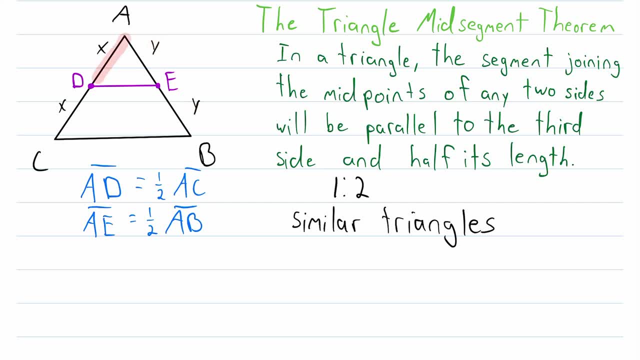 has a length of Y plus Y or 2Y. So now we've got two sides in these two triangles that are proportional. Then if we could show that the included angles of these sides in the two triangles are congruent, we could. 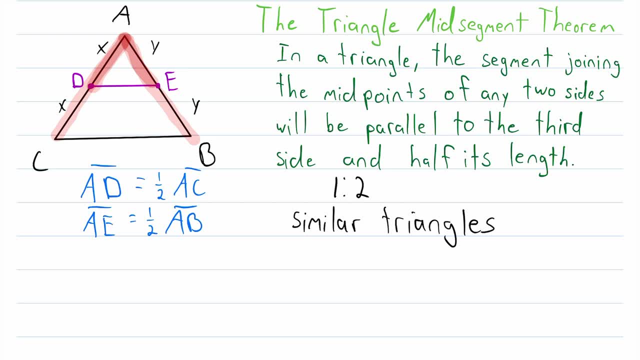 use the side-angle-side similarity postulate to conclude that the triangles are similar. Now, what's the included angle of the sides AD and AE? Well, that would be this angle. A right here. What is the included angle of the sides AC and AB? Well, that is also the very same angle. 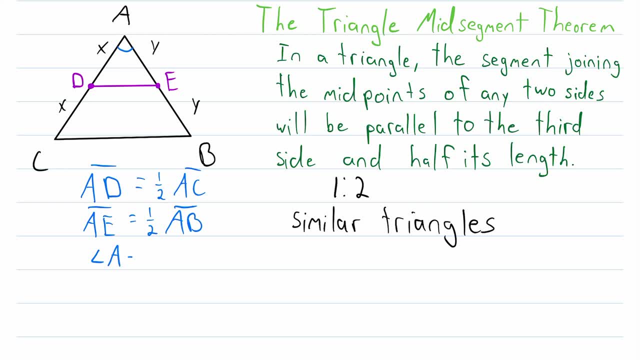 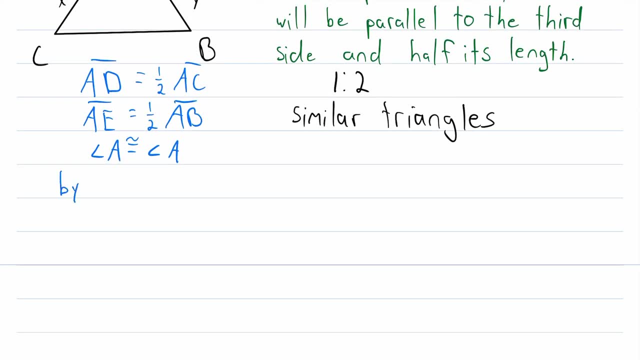 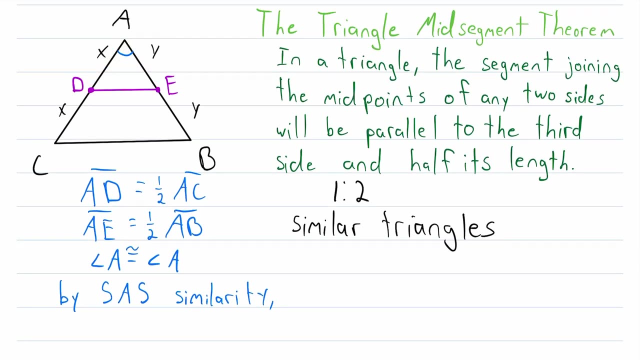 angle A. So we have, by the reflexive property of congruence, that angle A is congruent to angle A And therefore, by the side-angle-side similarity postulate, we can conclude that triangle AED is similar to triangle ABC. Now why is this so important? Why is this? 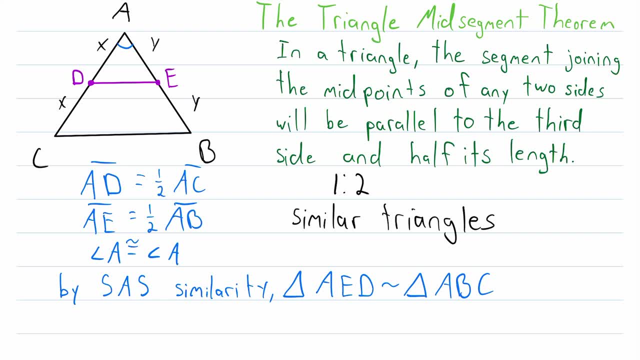 useful. Well, remember that corresponding sides of similar triangles are proportional. Since these two triangles are similar, and we know that AD is half the length of the corresponding side AC, we also know that DE is half the length of its corresponding side, CB. So isn't that cool? We'll say that DE has a length of Z. Therefore, CB has a length. 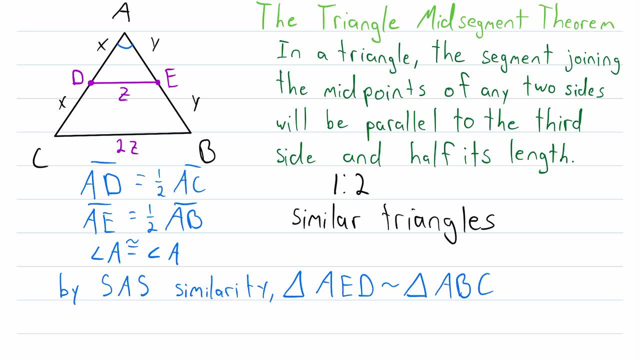 of 2Z Halfway done. we've proven one part of the conclusion that this segment joining the midpoints of two sides of a triangle is half the length of the third side of the triangle. Now we just need to prove that this segment, DE, is parallel to the third side of the triangle. 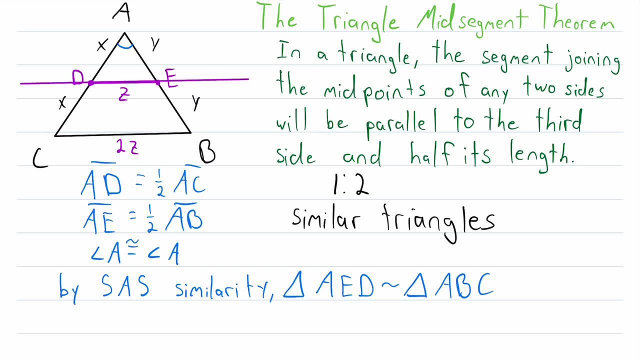 CB We say that two line segments are parallel. if the lines that contain those line segments are parallel, So a reasonable thing to do would be to draw these two lines that can contain the line segments we're concerned with. Then if you've worked with problems, 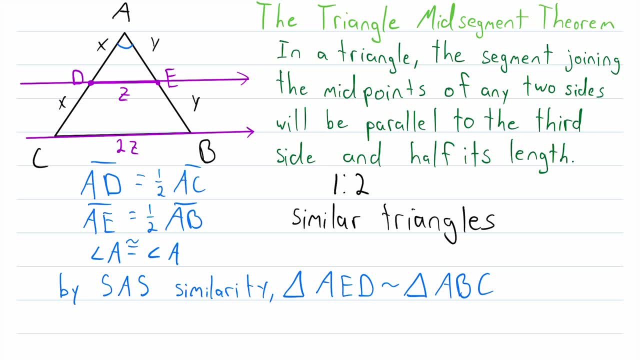 involving parallel lines. you might immediately notice something. These two lines are being cut by this transversal. They're also being cut by this transversal, but we can focus on just one. Let's focus on this transversal AB. 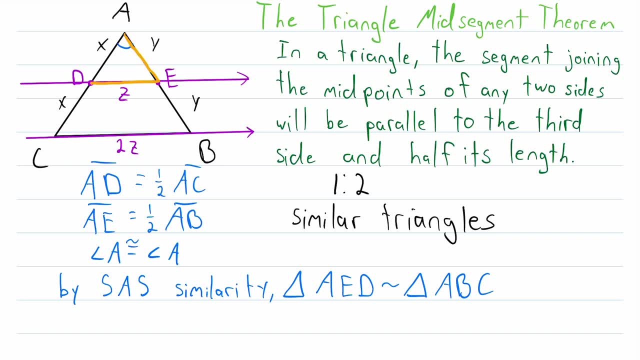 We see here this angle AED and this angle ABC. these are corresponding angles And if we can prove that these angles are congruent, then by the converse of the corresponding angles theorem we will have proved that these two lines are parallel. 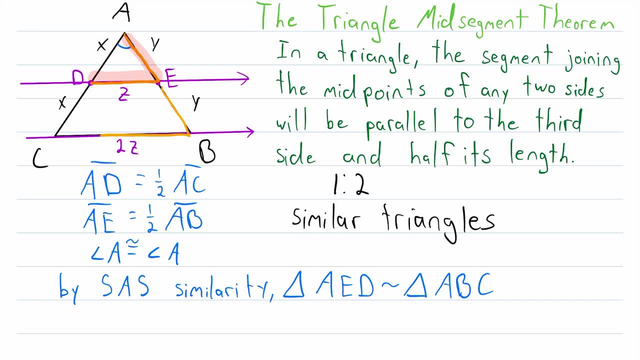 So are these two angles congruent? Well, yes, they are, Because, remember, similar triangles have congruent corresponding angles And the angle AED corresponds to the angle ABC. So, since they are corresponding angles in two similar triangles, the angle AED corresponds. 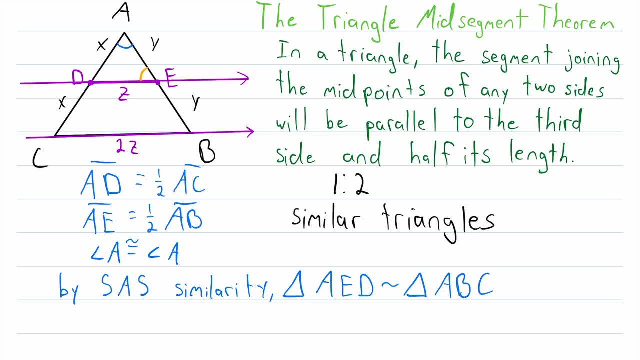 to the angle ABC. The angle AED is certainly congruent to the angle ABC And therefore by the converse of the corresponding angles theorem, since a pair of the corresponding angles created by the transversal AB are congruent, we know that these two lines are parallel And thus,